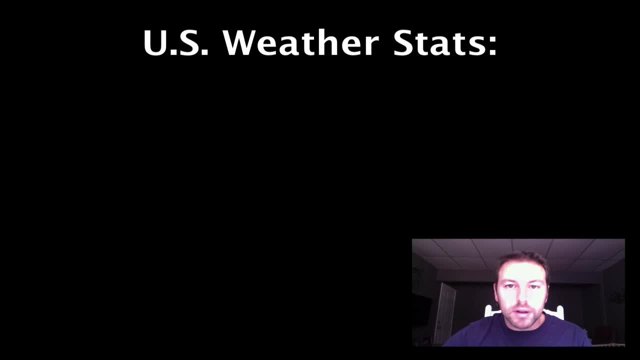 that you might want to be familiar with. You're not. you don't have to commit them to memory, but they're definitely pretty interesting. Some things like the hottest in Death Valley, California, over 100 or about 134 degrees Fahrenheit. Coldest, Prospect Creek camp in Alaska- negative 80 degrees. 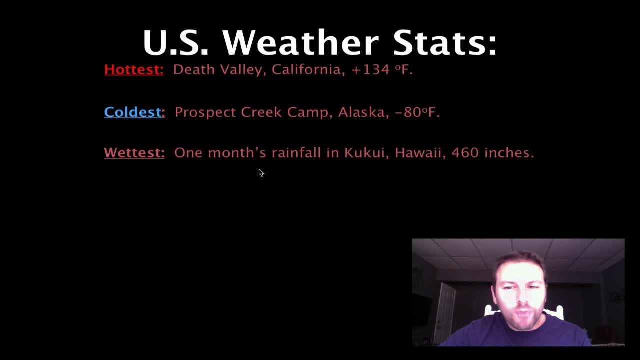 Fahrenheit. Okay, wettest in Hawaii: 460 inches of rain in one month. Actually, right now, Long Island, I think we're a couple inches down from normal and I think we get around 10 inches of rainfall roughly around this time of year, and California has gotten- I mean- sorry, Hawaii- 460 inches of one. 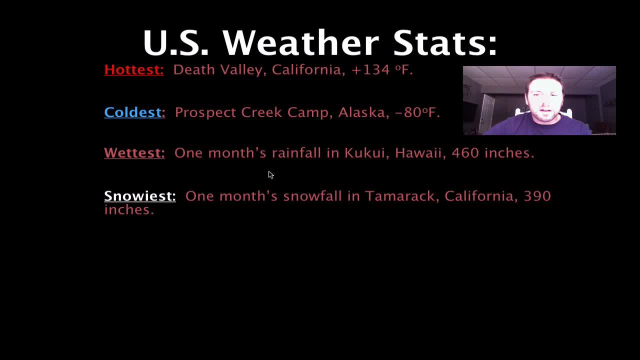 in one month. Pretty amazing. Snowiest in California: 390 inches of snow for a month. Dryest in Baghdad, California. once again another California place: 767 days without rain And windiest. we're looking at a Mount Washington, New Hampshire, just a little north of us, with the highest winds recorded at 231 miles per hour. 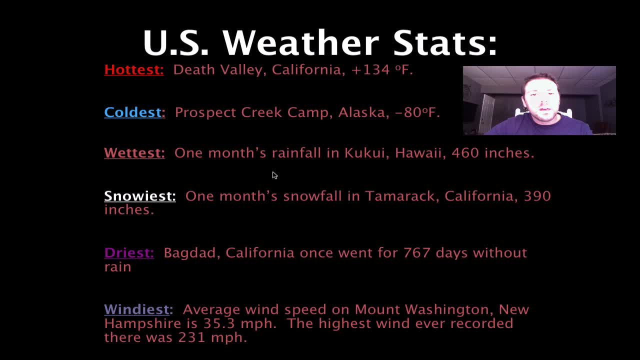 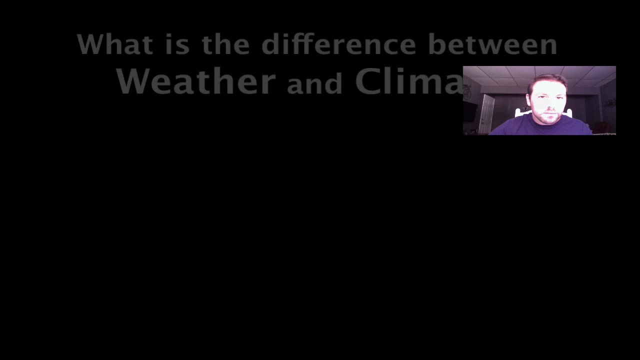 Those are well over hurricane force winds, and you're looking at winds that we typically see tornadoes. So there are definitely in within the United States, many, a huge number of extremes, from coldest to hottest, snowiest, and driest and windiest. It's actually pretty amazing. Okay, so what is the difference between weather? 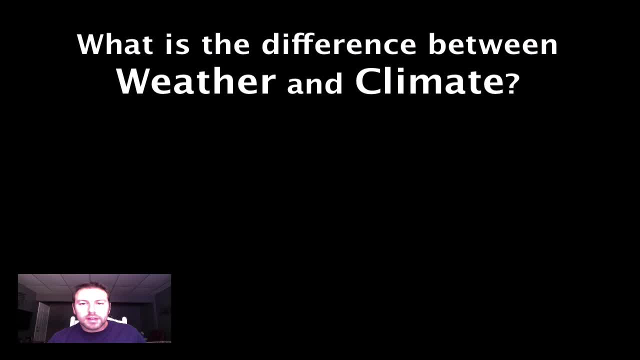 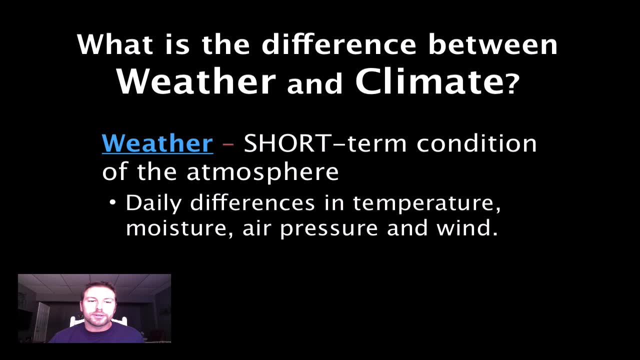 and climate. We commonly hear these terms being used and here we have a little definition for it. Weather is our short-term conditions of the atmosphere. Okay, daily differences in temperature, moisture, air pressure and wind, along with a couple other variables. So you're looking. they. 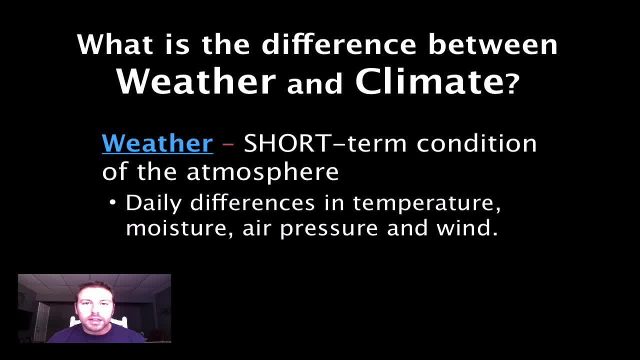 can change from hour to hour, Day to day and season to season. Climate, on the other hand, is our long-term conditions. What's our climate been like for the past two years, three years or over the past 10 years? So weather is our short-term climate, is our long-term conditions. 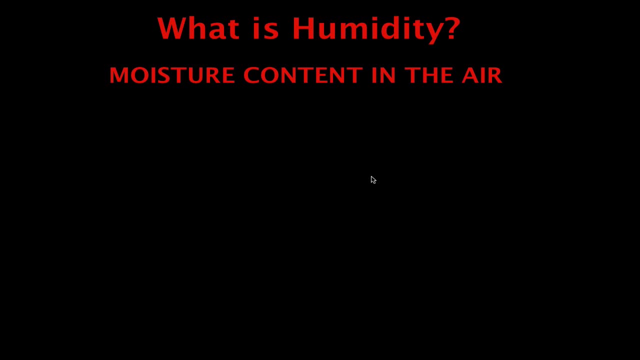 One of the first weather variables that we're going to be looking at is humidity. Humidity is the moisture content in the air. We can look at humidity in a couple of different ways. The first one is humidity. Humidity is the moisture content in the air. We can look at humidity in a couple of different ways. The first one is humidity. 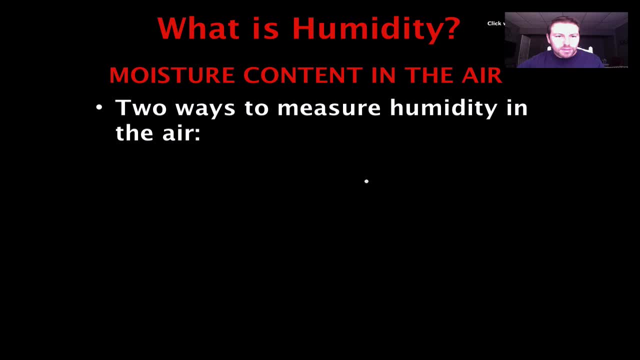 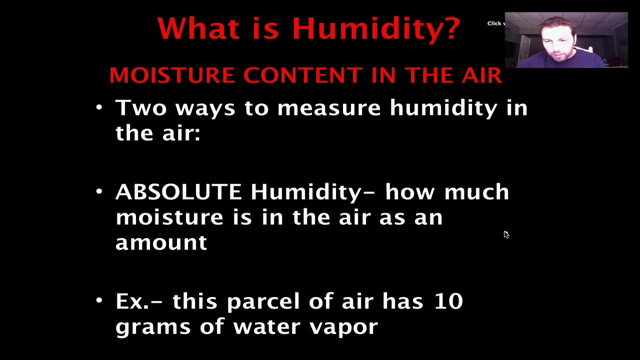 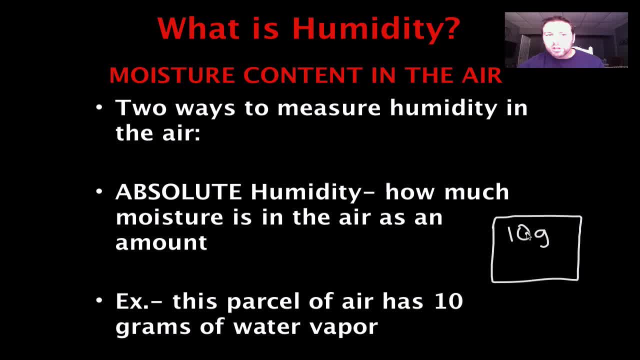 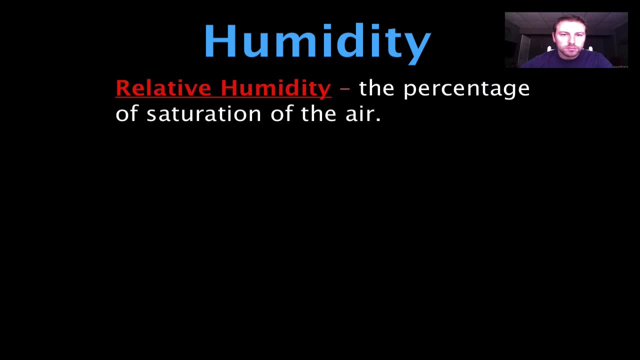 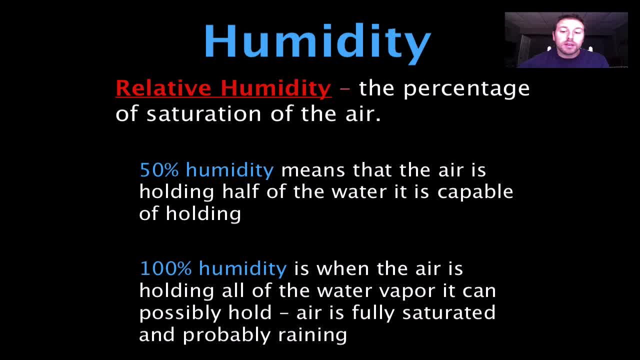 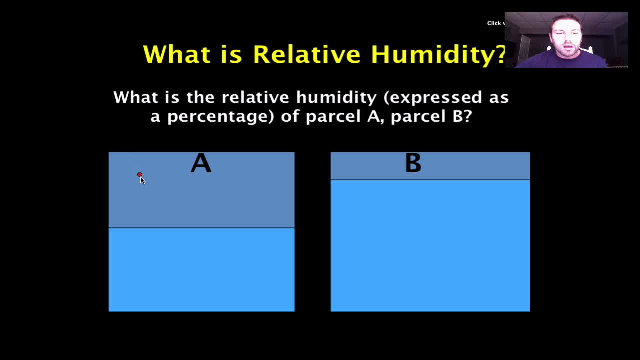 humidity in a couple of different ways. The sixth one is humidity. Humidity is the moisture content in the air. We can look Humidity is the moisture content in the air. We can look 100 grams. you get 50 percent on parcel b. parcel looks about the same 100 grams. but now our dark 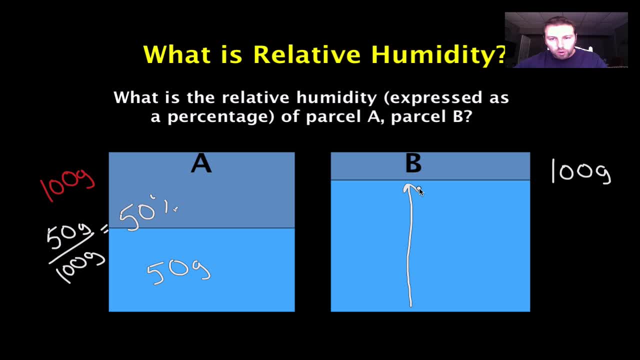 blue region has increased. it's more. we'll write. we'll say: this is about 80 grams of water. so now parcel b. we could do the percentage 80 over 100 grams to get our 80 percent. so parcel b is filled with more water. so when it's filled with more water the relative humidity goes up. we can also 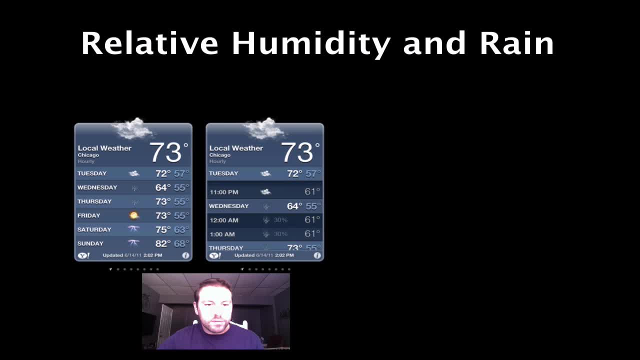 look at relative humidity and the chance of rain. we have two screencast screenshots right here and we can see local weather in chicago, 73 degrees, and looking down through you see that there's some rain appearing. Same thing: we could look at the hourly thing. 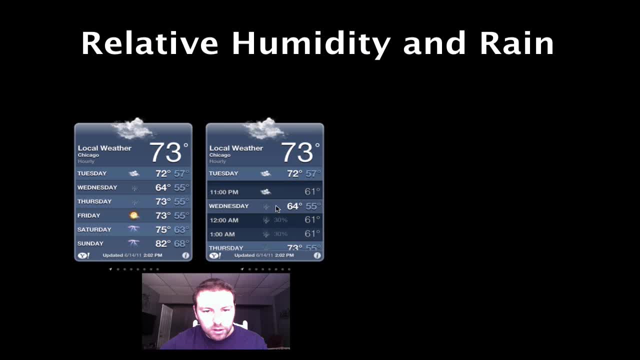 Tuesday: 72 degrees for the highs and lows, but we also see rain. There is a correlation between relative humidity and rain. As the relative humidity increases, the chance of precipitation also increases, and that would have a tendency to make sense, As there's. 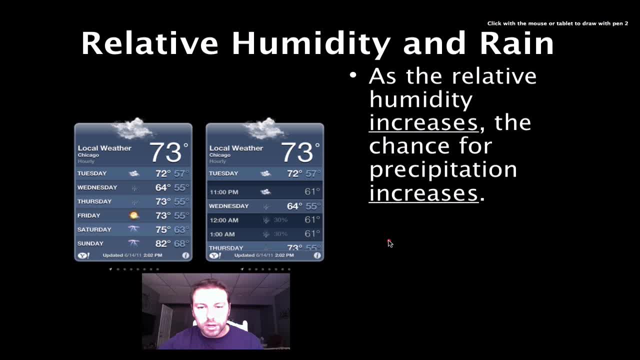 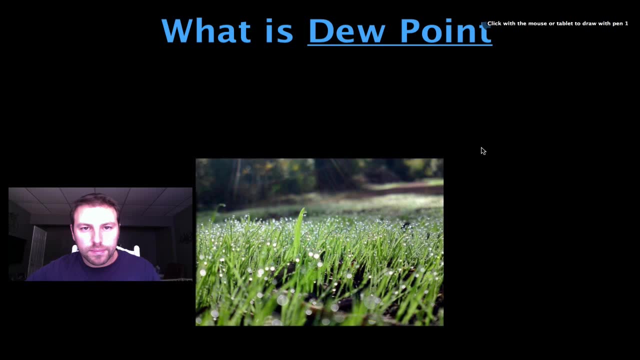 more water vapor in the air, we potentially could have more rainfall. An example would be 90% humidity, relative humidity- very high chance of rain. Another term we're going to have to be familiar with is the dew point. The dew point is the temperature at which air is holding the maximum amount of water vapor. 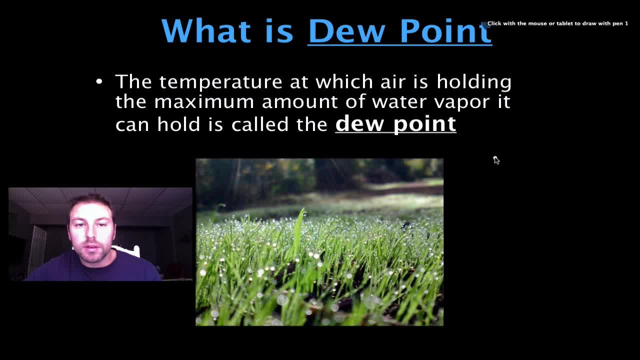 it can hold. So, for instance, if maybe the dew point temperature is 12 degrees Celsius and the air temperature reaches 12 degrees Celsius, then the dew point temperature reaches 12 degrees Celsius and the air temperature reaches 12 degrees Celsius, and the air temperature reaches. 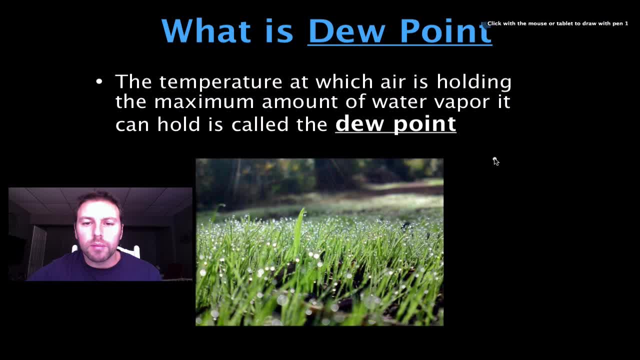 12 degrees Celsius. the air will now become fully saturated and the air temperature has reached its dew point. It cannot hold any more water. This image down here in the bottom we often associate: like during the summer we see dew on the grass. What happens is during the 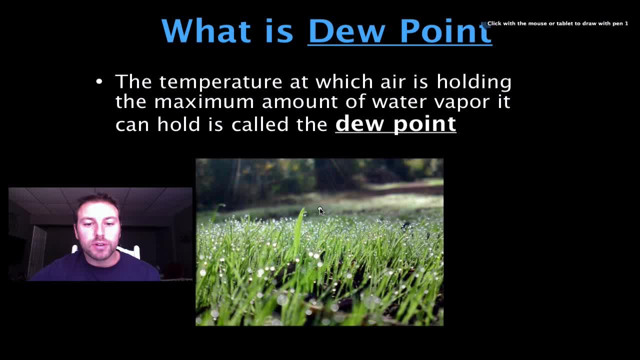 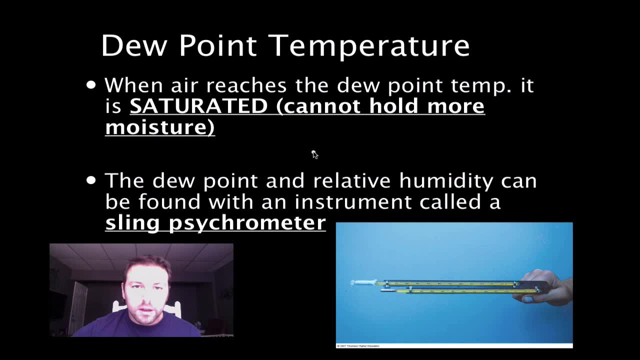 night, the temperature is dropped, making the air more saturated, and the water ended up condensing on the grass. Like I said earlier, the dew point temperature is at which air is fully saturated and to how much it is condensationous. during the day That will also be. Indica claim means that 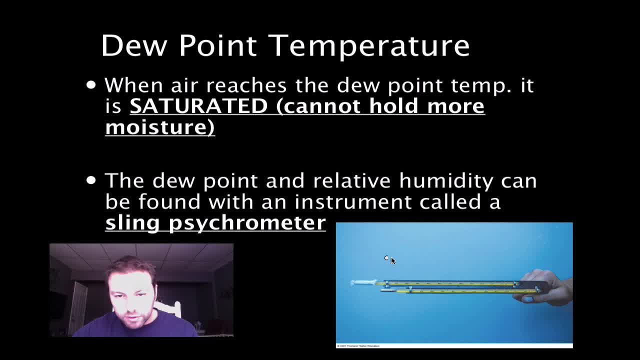 necessarily, and it will also mean the dew point temperature drops. On the other hand, something else that even could happen with wet climates is that the dew point meat isТ saturated. We can find this dew point temperature using what's called the sling cyclometer. this sling cyclometer looks like this device right here. 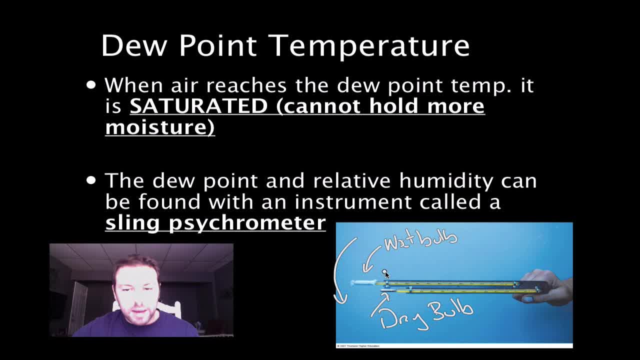 we sling the whole thing around And what ends up happening is by finding the differences in the temperature between the wet bulb and dry bulb. we're actually able to find the dew point temperature using a chart that's in our reference table. Here's a little cartoon. 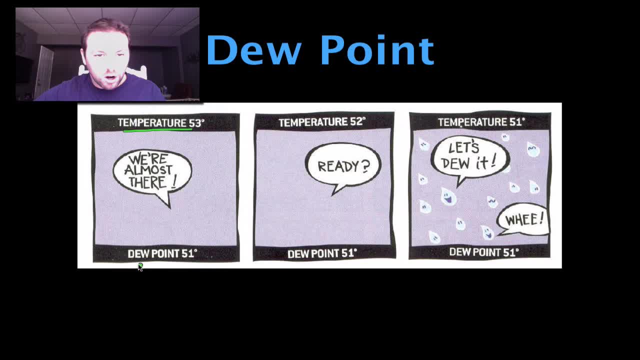 So we have the temperature: 53 degrees. Our dew point temperature is 51. And this is our parcel of air right here. And notice there something in the air saying we're almost there. Temperature drops, It's going down from 53 to 52 degrees Dew point temperature. notice it stays the same. 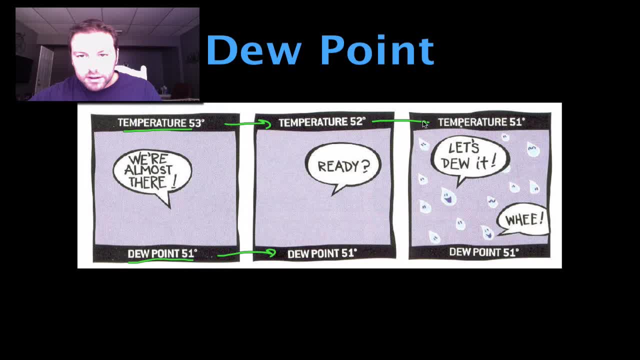 We're getting ready. And then, finally, when the air, when the temperature, reaches our dew point temperature, let's do it- It begins to rain. So here, as our air temperature reaches our dew point temperature, relative humidity, Humidity is increasing, And here it finally increased so much the air became saturated and 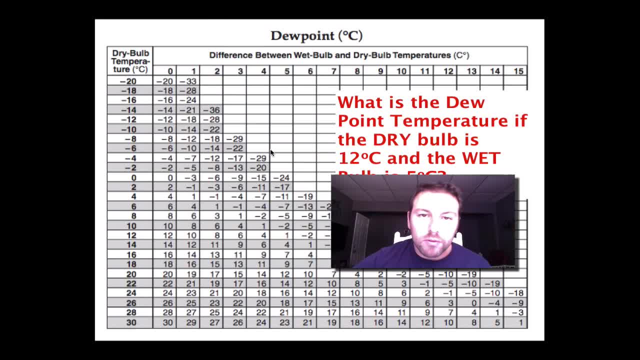 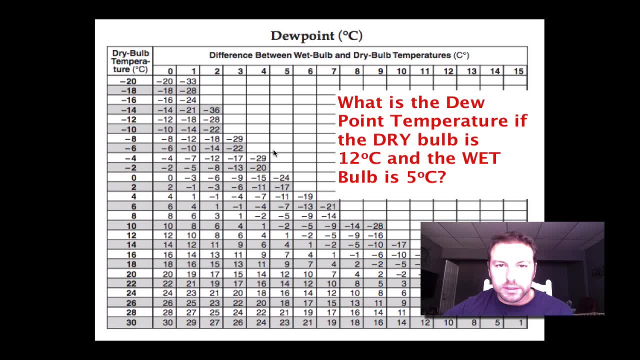 it rained. If we open up our reference table, we can find our dew point and relative humidity chart. The dew point- relative humidity chart is used with the sling psychrometer. Remember the sling psychrometer has a wet bulb and a dry bulb, From the difference between our wet bulb and dry bulb. 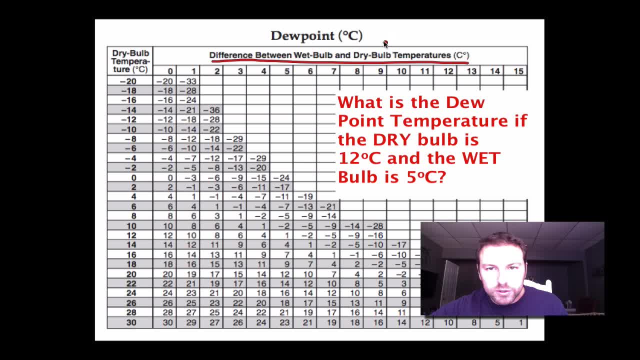 right here on the top. okay, difference means we subtract wet minus dry And using our dry bulb temperature on the from the sling psychrometer, which is the same as your air temperature, we're able to find our dew point and relative humidity. So an example would be: 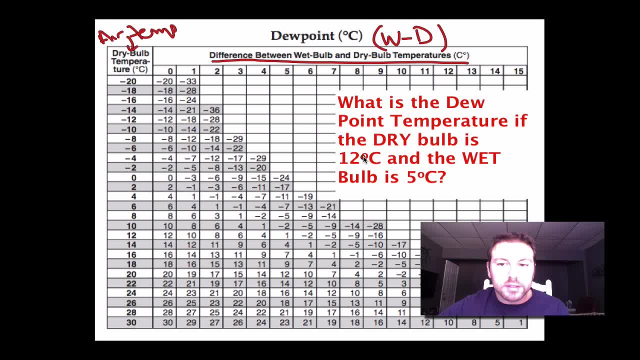 what is the dew point temperature if the dry bulb is 12 degrees Celsius and the wet bulb is five degrees Celsius? Well, first we go to left side and we find our dry bulb temperature. So we're able to find our dew point and relative humidity. So an example. 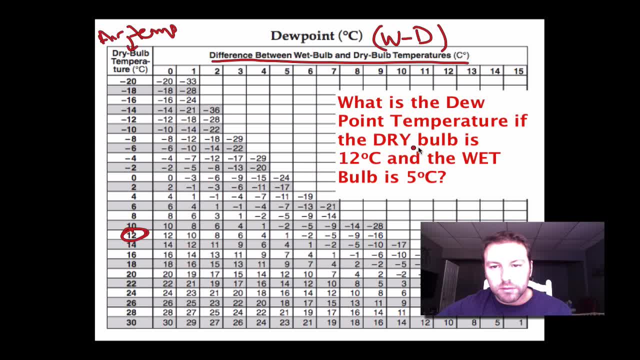 of that is our dew point temperature or our air temperature. Then what we need to do is we need to find the difference between our wet bulb and our dry bulb. So 12 minus 5 equals 7.. So we go up to the top, we find 7, and where the two numbers meet is our dew point temperature. So here, 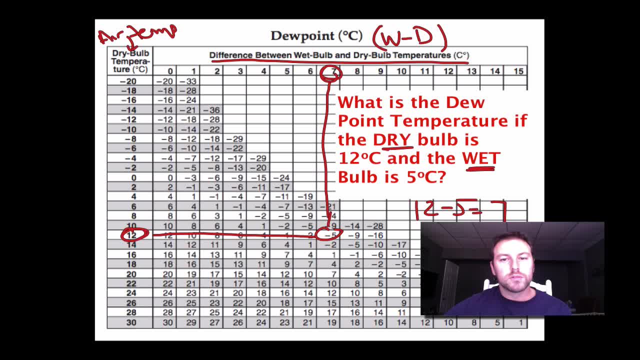 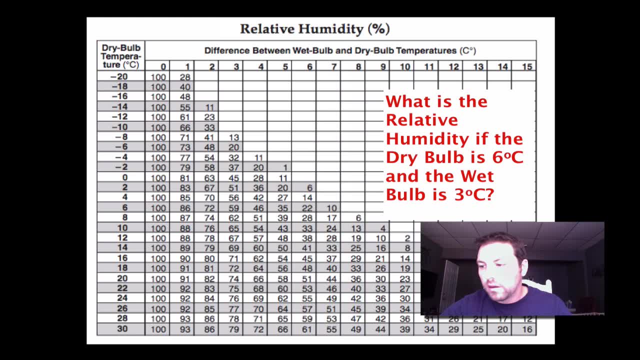 dew point is negative, five Done, Pretty easy. We can do the same thing over here. So our dew point temperature, our dew point is negative, five Done, Pretty easy. We can do the same thing over same exact thing to find our relative humidity. Using the sling psychrometer we can also find: 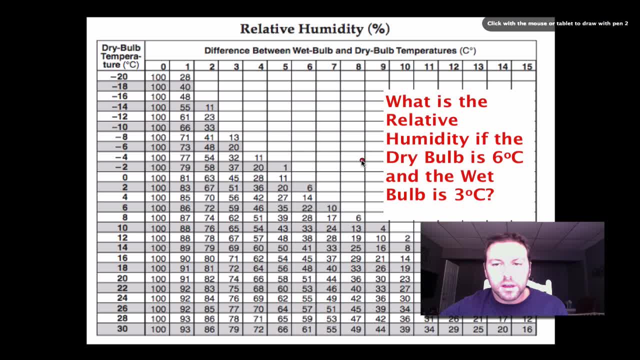 the relative humidity. We can do the same exact procedure we did before. So we need to know our dry bulb and we need to know our wet bulb. So we go to the left side, look for our dry bulb temperature of six degrees Celsius. Then we need to find the difference. 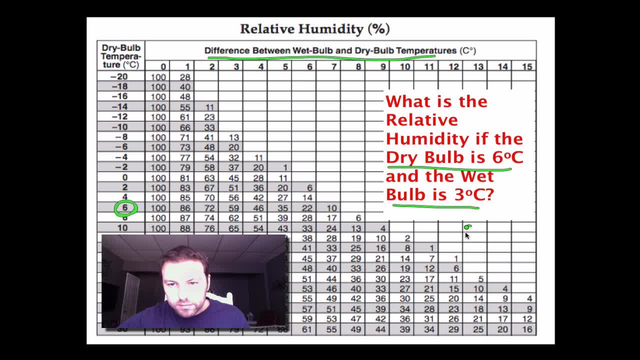 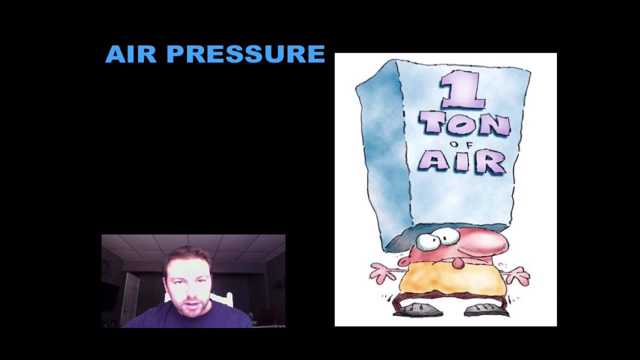 between the wet bulb and dry bulb. Six minus three equals three. Find three on the top and we're going to move down to where we both hit. and there you go. 59%, Same exact procedure for using dew point and relative humidity. All right, we're going to stop here for this screencast. We've 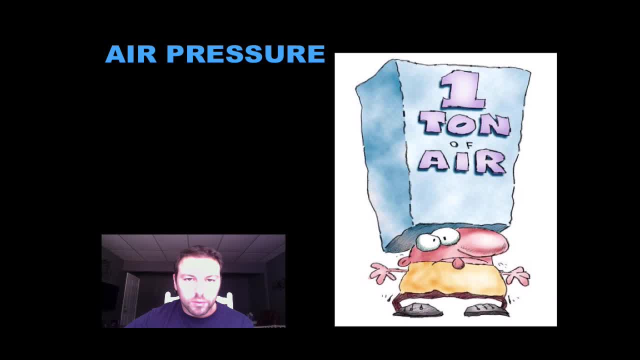 covered a lot between relative humidity and using the sling psychrometer with the relative humidity Dew point charts. Next time we start, we're going to go into air pressure.